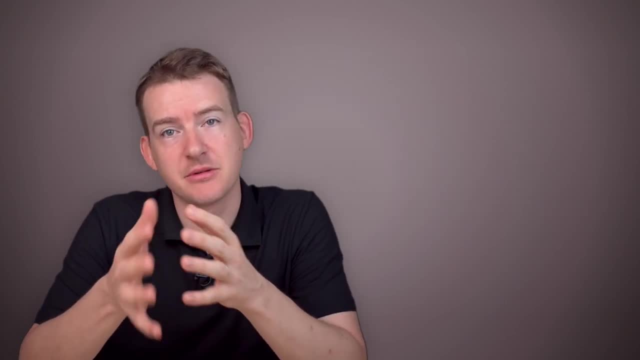 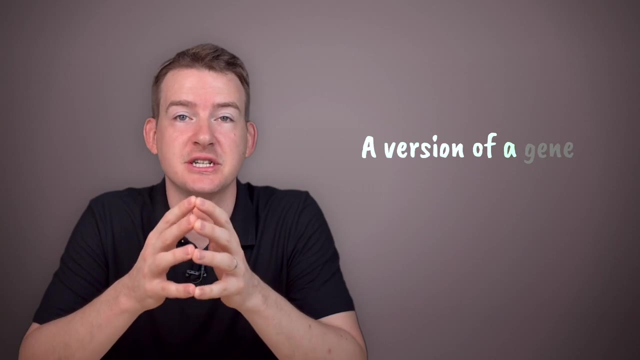 The reason that you are unique, the reason that people are different from each other despite having different genes, is that genes come in different versions. A version of a gene is known as an allele. For example, there are several genes that determine what eye colour you will have. 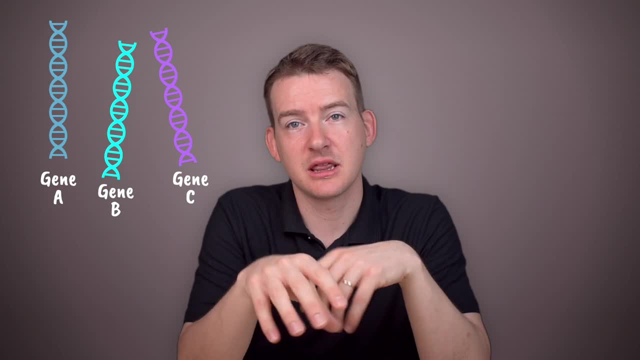 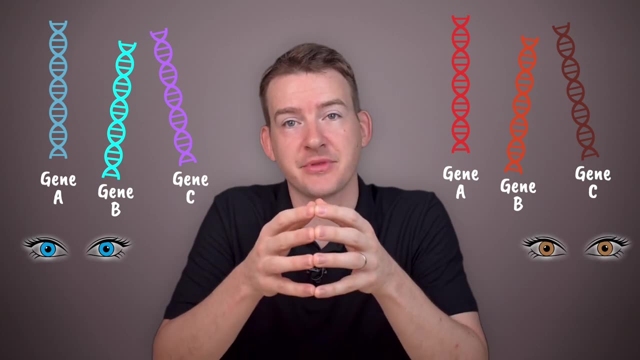 If you have one set of alleles for those genes, then you would have one eye colour, But if you have different alleles for those same genes, then you would have a different eye colour. It's the same genes for everyone that determine eye colour, but different people have different versions of those genes. 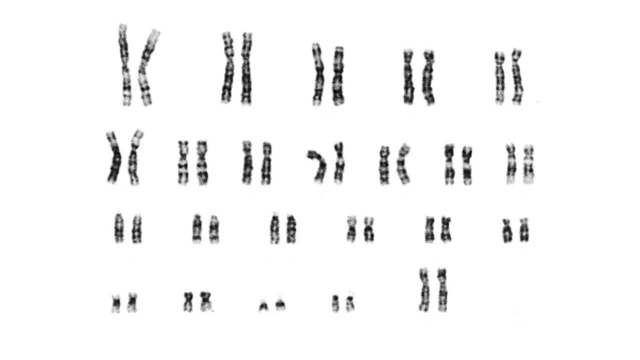 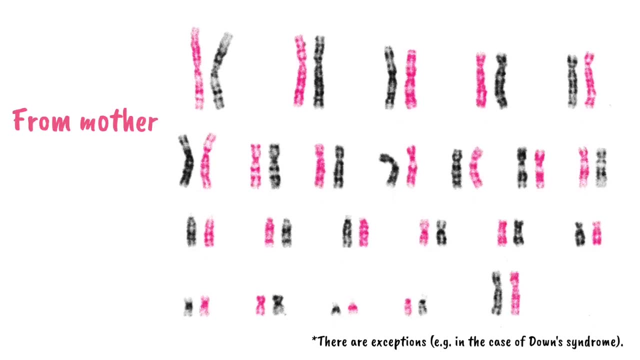 Hence different features. Humans have 23 pairs of chromosomes, totalling 46 chromosomes, in their cells. They get 23 chromosomes from their mother and 23 from their father. Since each person inherits two sets of chromosomes, one from each parent, this means they inherit two of every gene. 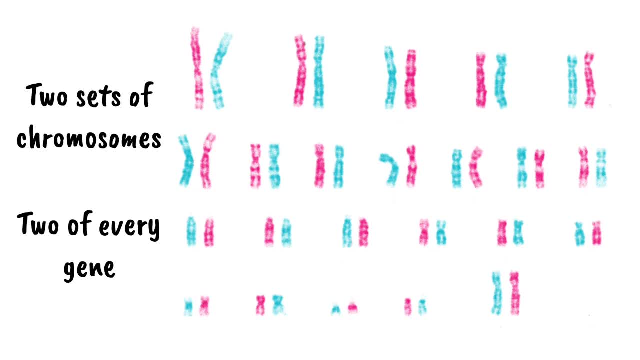 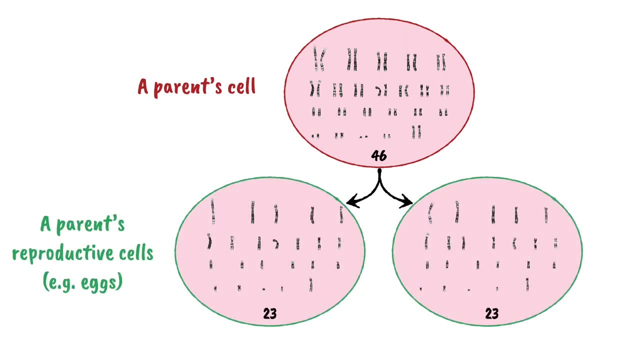 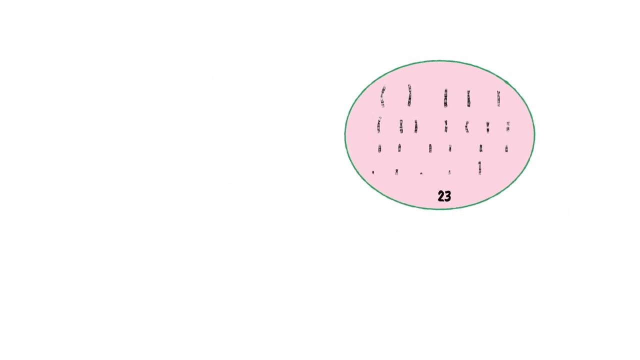 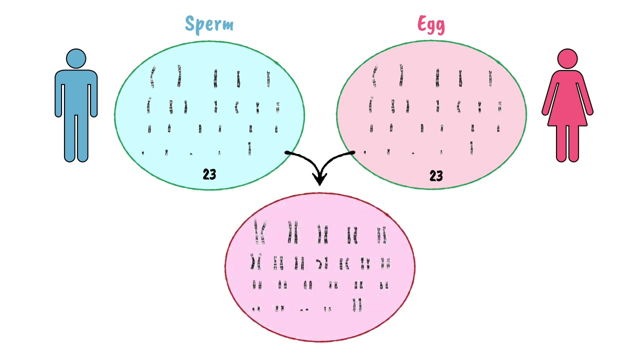 When reproductive cells are formed, for example egg cells, some of the parent cells with 46 chromosomes divide in a way to provide reproductive cells, each with 23 chromosomes in them. Each sperm cell and each egg cell contain 23 chromosomes so that when they combine they produce a new cell. 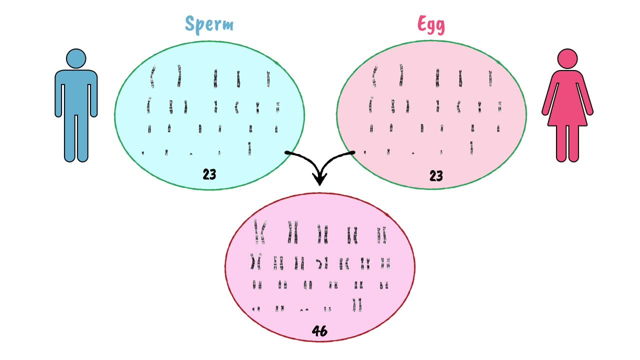 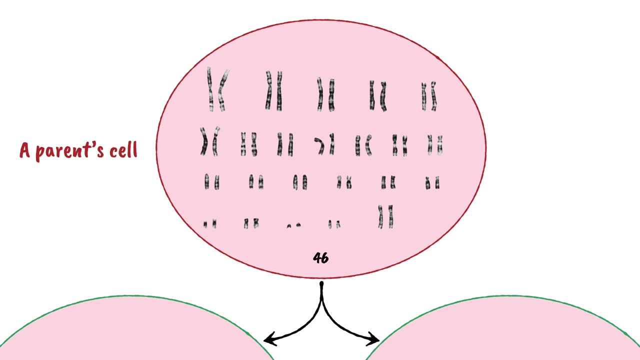 The new cell has the correct number of chromosomes, and that cell divides and develops to become a new human. When reproductive cells are produced in the parents, exactly which one of the pair of chromosomes will be passed on is random. Remember that chromosomes contain genes. 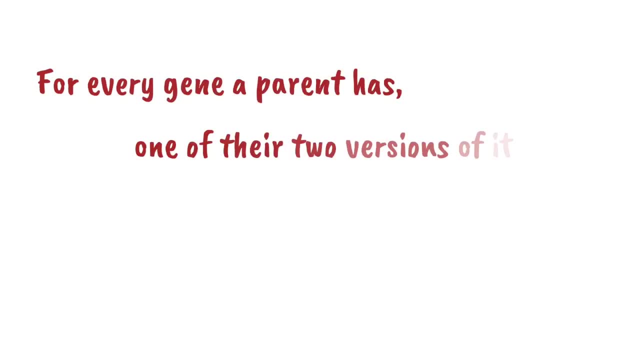 For every gene a parent has, one of their two versions of it is randomly passed on to their child. Let's look at the inheritance of a specific trait to understand what this might mean in real terms. There is a genetic disease called cystic fibrosis. 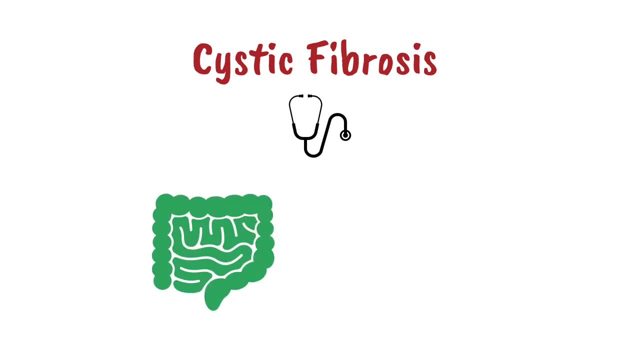 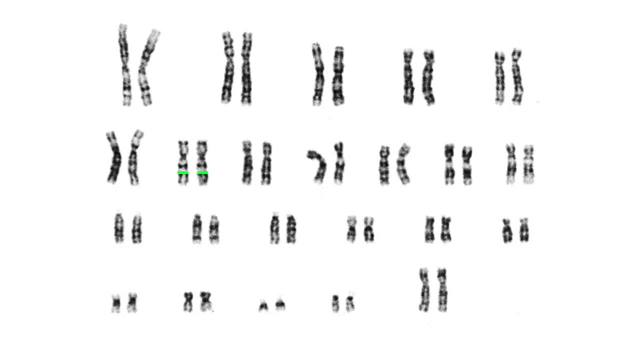 that causes the body to produce sticky mucus in the digestive system and lungs. This causes problems with digestion as well as lung infections. There is a gene found on chromosome 7 which codes for cystic fibrosis, and most people express a version or allele for this gene. that is normal, meaning they don't have cystic fibrosis. 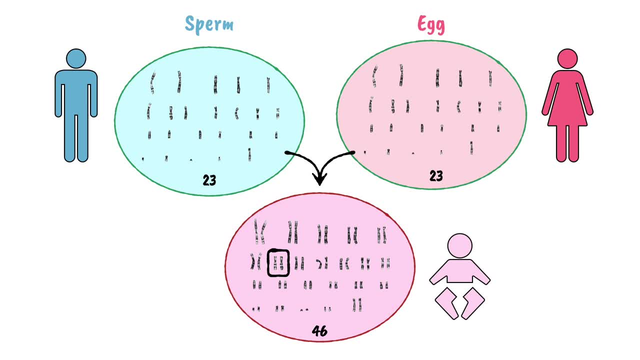 Remember that a baby will inherit two versions of chromosome 7, one from each parent, just like all chromosomes, And therefore will inherit two copies of this cystic fibrosis gene. Let's focus just on this gene within a person's cells and let's use some symbols for it. 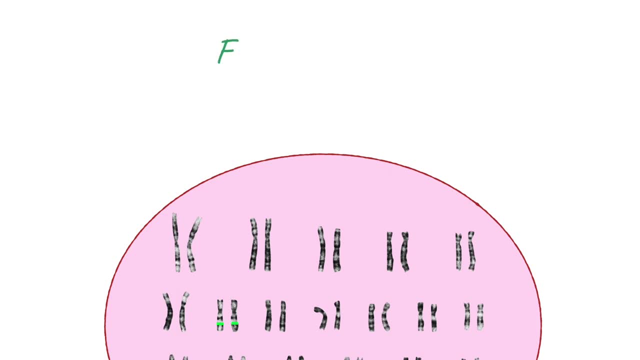 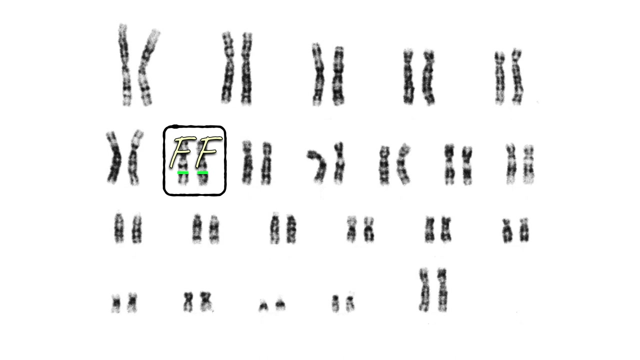 We usually use letters of the alphabet, so let's go with F for fibrosis. We'll say that uppercase F represents the normal version of the gene and lowercase f represents the version of the gene that codes for cystic fibrosis. Most people have two normal alleles of this gene. 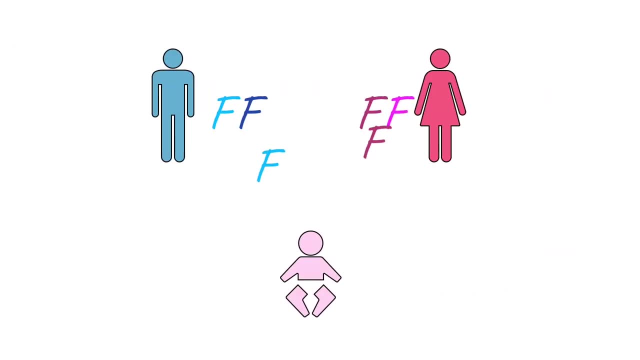 and so whichever one of their two alleles each parent passes on, their baby will have two normal alleles. But let's look at other possibilities. Let's say both parents have one normal allele and one cystic fibrosis allele. It's possible the baby may by chance inherit this version from their father and this one from their mother. 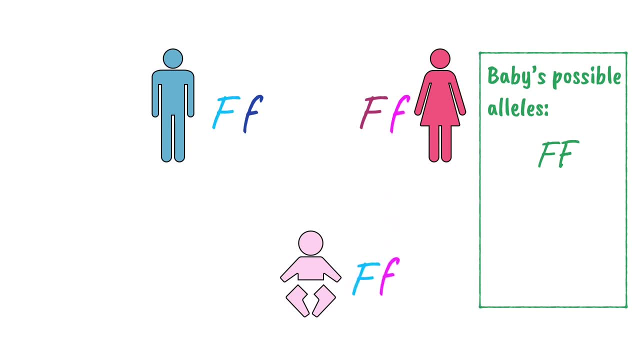 They may instead inherit this version from their mother and have one normal version and one cystic fibrosis version. They may instead inherit a normal version from their mother and a cystic fibrosis version from their father, Or two cystic fibrosis versions, one from each parent. 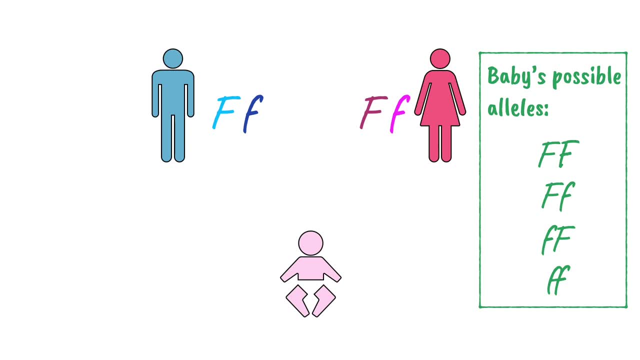 As you can see, there are four different possibilities of inheritance. By the way, if we look at this possibility, we tend to write the uppercase letter first, so this combination would usually be written like this: So what do these combinations mean in practice for this baby? 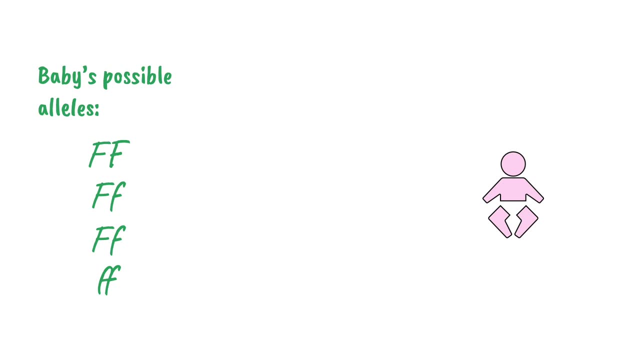 Remember that uppercase F is our symbol for normal or doesn't have cystic fibrosis. So if the baby were by chance to inherit this combination, they would not have cystic fibrosis. Lowercase f represents the cystic fibrosis version, and if the baby inherited this combination, they would suffer from cystic fibrosis. 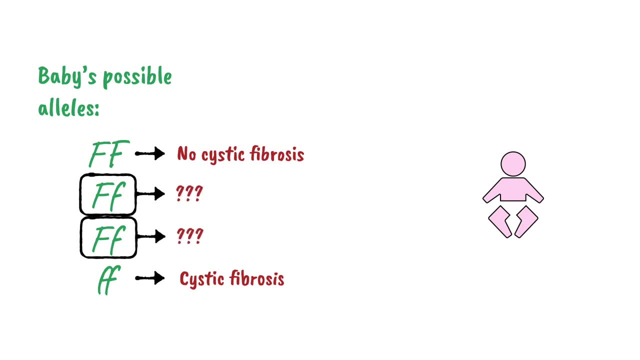 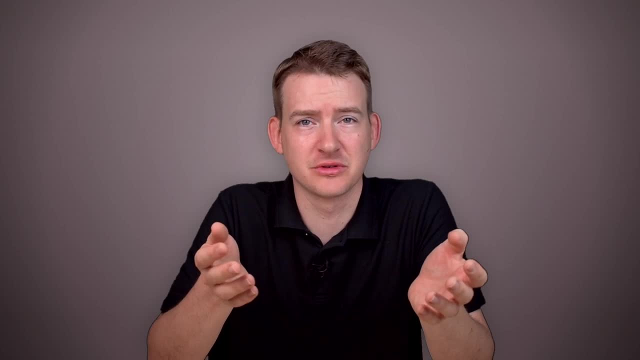 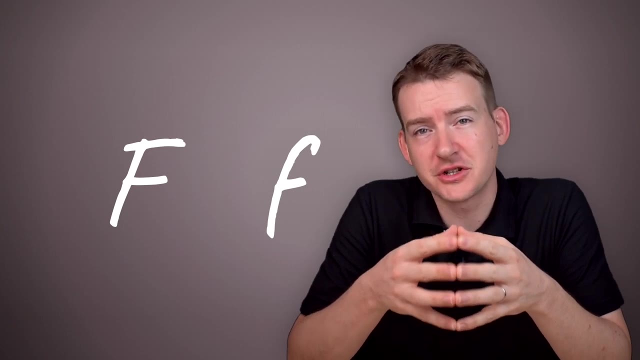 But what about a child who inherits both alleles? There are only two possibilities here. The child either has or does not have cystic fibrosis. So which one is it? Well, in the case of this gene, like with many genes, one version of it is kind of stronger than the other one.